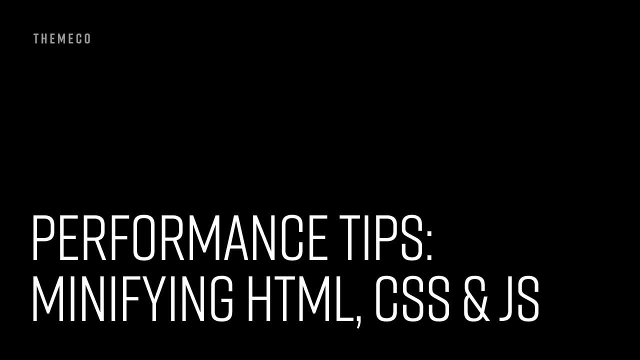 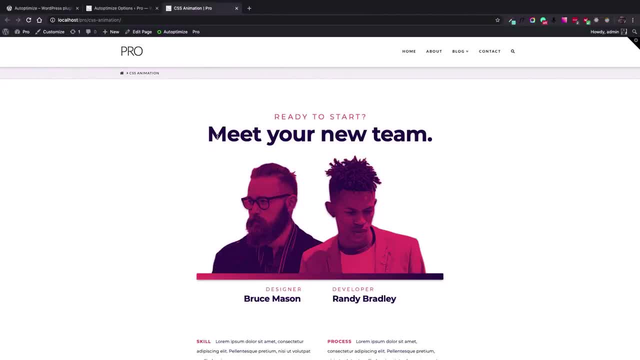 Hi everyone, Christopher here from Themeco with another video from the performance series. Today we are going to discuss how to minify and merge your assets of your web page, including the JavaScript files and CSS files. I am going to use a plugin called Auto Optimize in this video, which. 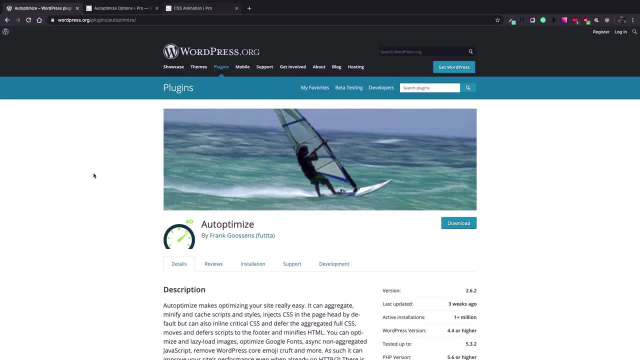 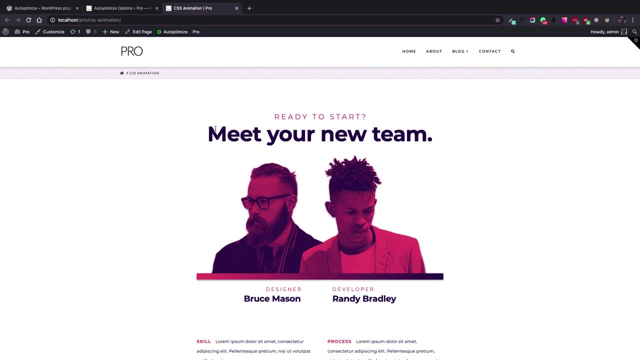 has a free version that you can download from the wordpressorg official website, but it is somehow a subjective issue and you can use many different plugins that are available Both in a free and paid versions, and you can use whichever plugin that you feel it will do the best. 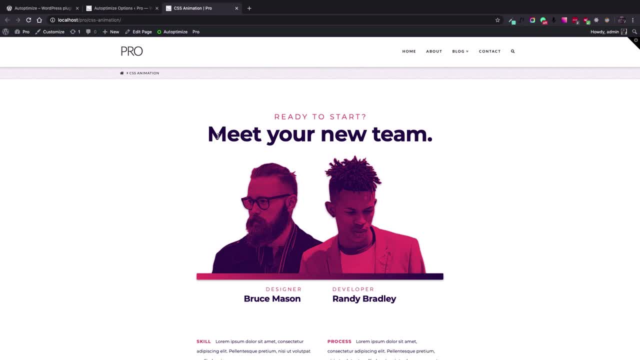 for your case scenario. But in this video we are going to use the Auto Optimize plugin and try to set some options of the plugin to make sure that we can minify and merge our website assets and make it much more faster than the original version. So let's get started. 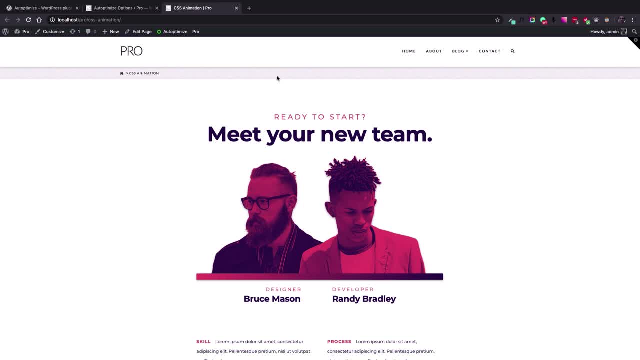 I have a page on my website with a simple header at the top with the sub menus and menu items and also one of the design cloud content. So it is a simple page that we are going to make sure that the assets of the page are minified and as quick as possible to load, To make sure that I have all the assets at hand and 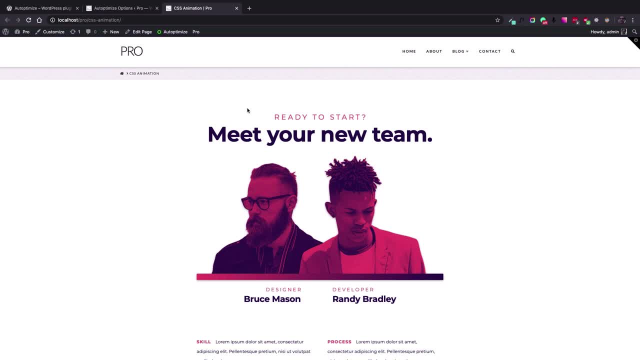 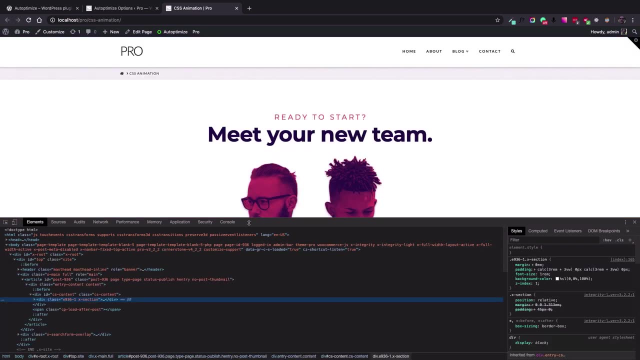 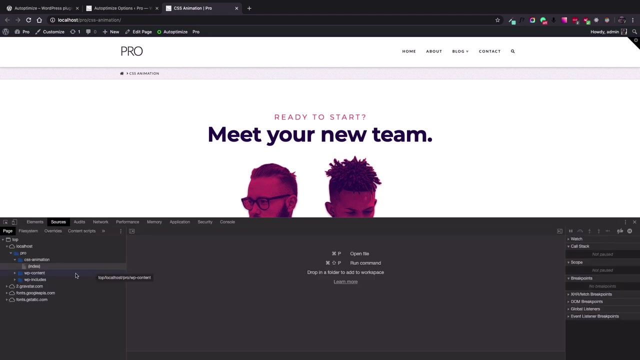 know what kind of JavaScript and CSS files are loaded in the page. I am going to use the Chrome Browser Developer Toolbar. I will right click on the page and select the inspect option to open up developer toolbar, and then I'm going to go to sources tab there. you can see that. 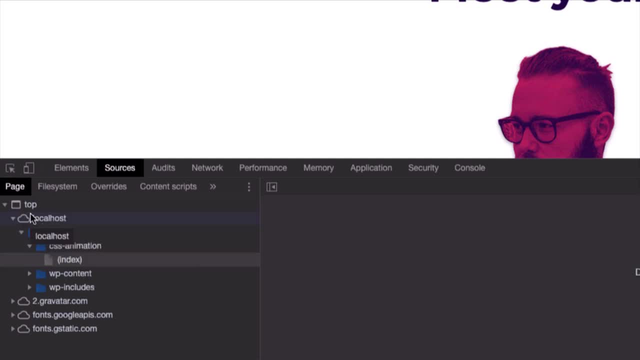 we have the address of all the assets that are available on the page and if I go to pro WP content, which is the WP content folder of a WordPress installation, you can see that there are two folders: plugins and the pro theme folder. in the plugins I have auto optimize plugin assets that I already 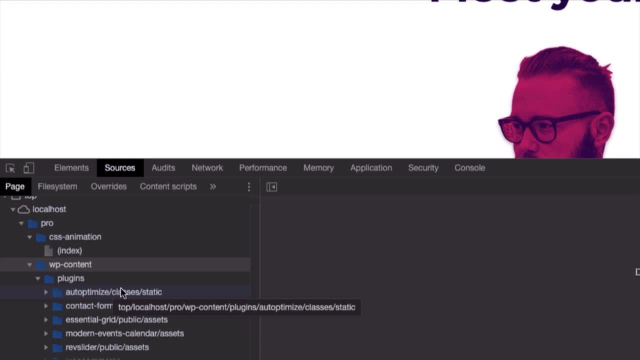 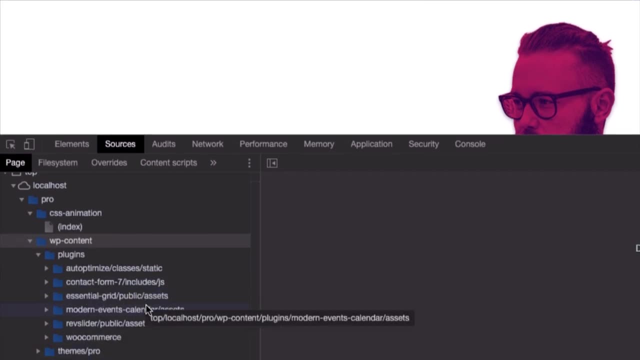 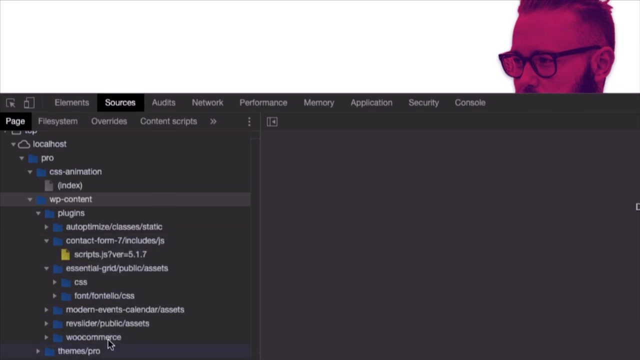 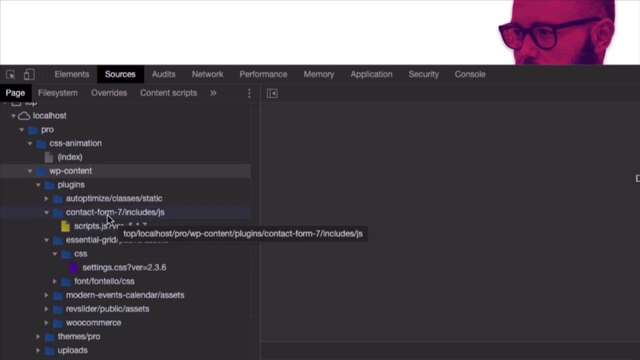 installed, but I did not set the settings and options of the plugin yet and we have the contact form, 7 essential grid and different plugins. each plugin has its own scripts or CSS files that are loaded in the page. in the previous video, I showed you guys how to make sure that you are going to load only the plugins that you 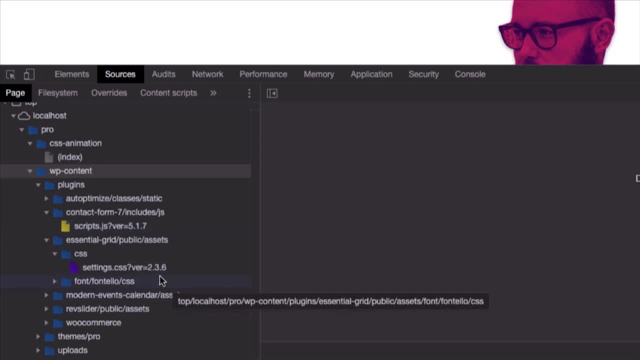 will need for the page, but in this video I'm going to show you guys how to just merge and minify all those files that you see now in the screen. this is important that in the themes folder, when you go to themes pro folder, we have few JavaScript files. 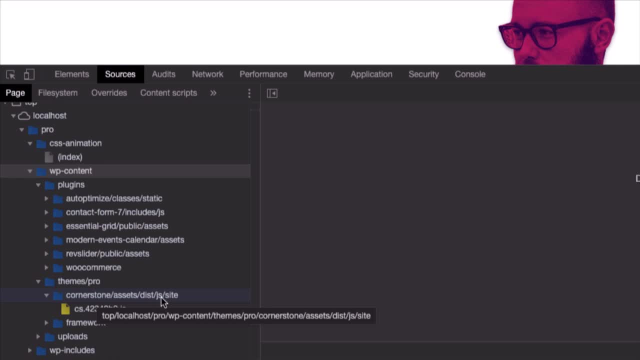 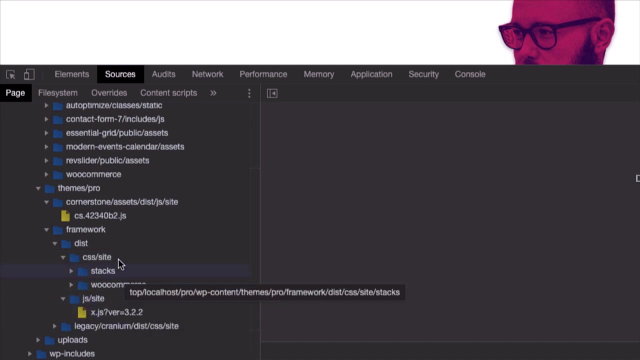 inside the cornerstone assets- distjs- site folder and the name of the JavaScript file is CS, dot and then combination of: I just numbers and characters. this is a JS file that is loaded in the page using our theme, and also we have a frameworks- framework folder with different CSS and JavaScript files available and loaded in the page. 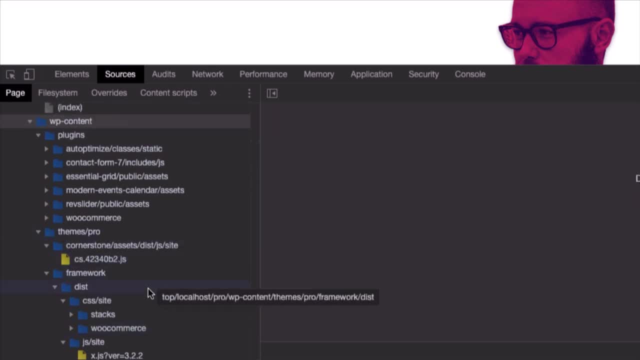 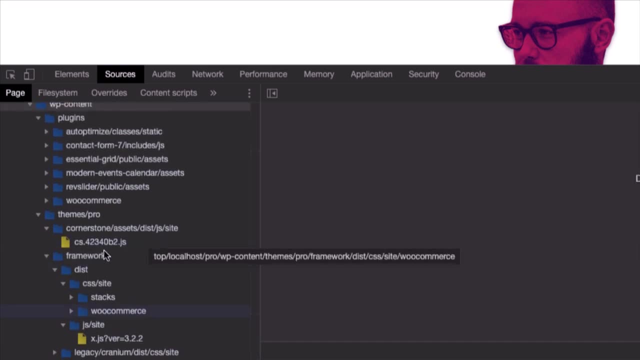 now why I show you guys the address of this files? because whenever we enable the settings and make sure that all the files are minified and merged using the auto optimize plugin, there might be cases that the front end of the website will stop work. So maybe the menu item does not. 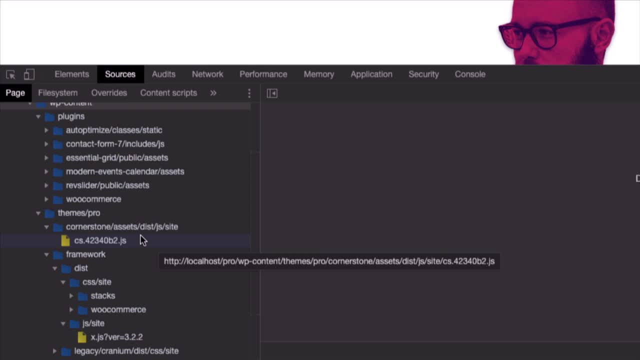 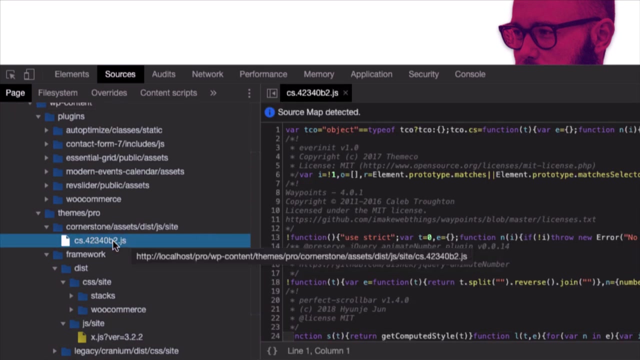 the sub menus does not show, or maybe there is a problem which shows that the JavaScript file is not loaded correctly. Our JavaScript files in the theme are already minified, So that is why we do not need to minify it again If we have double minifying feature. 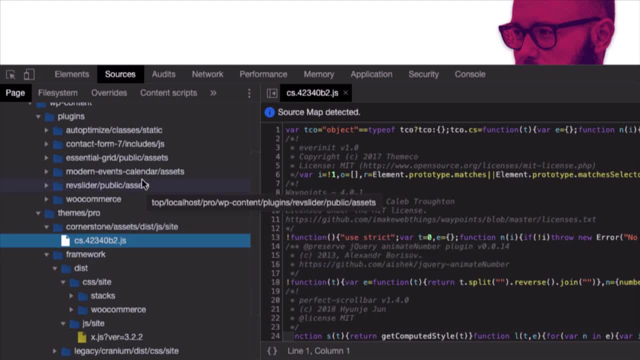 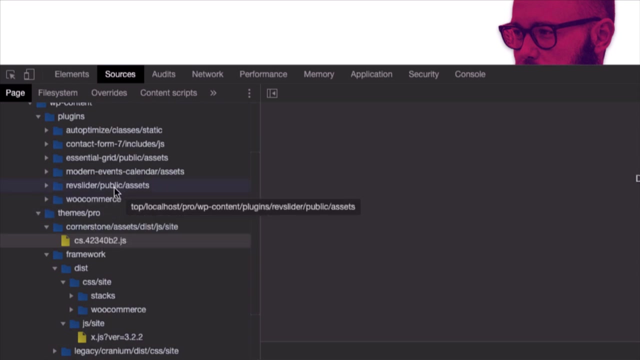 the file will be corrupt, But auto optimize plugin is clever enough to detect the already minified files to avoid the problem. but to make sure that we do the performance and auto optimize plugin set is correctly And we're gonna write down the URL address of this file. 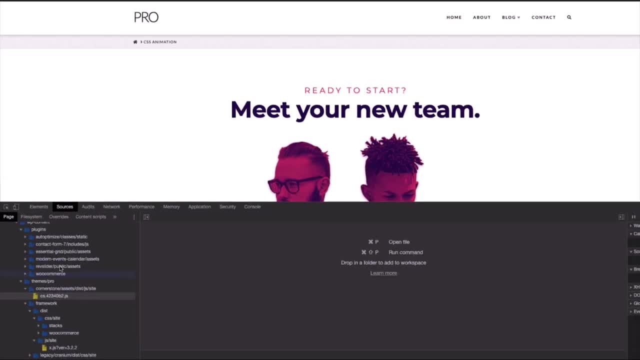 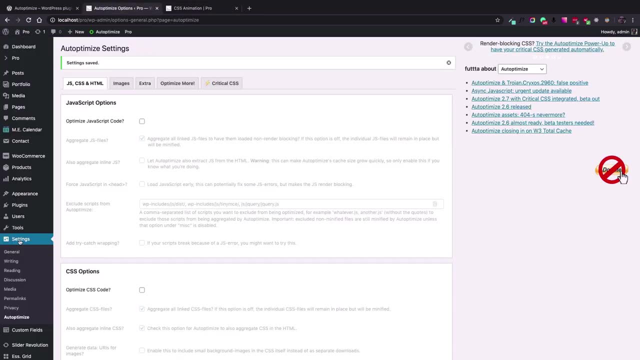 in case that there is a problem. So now let's go to the auto optimize options. To access the auto optimize options, you would go to the settings menu and the auto optimize menu, which is right below the item item, or you can click at the top of the admin page. 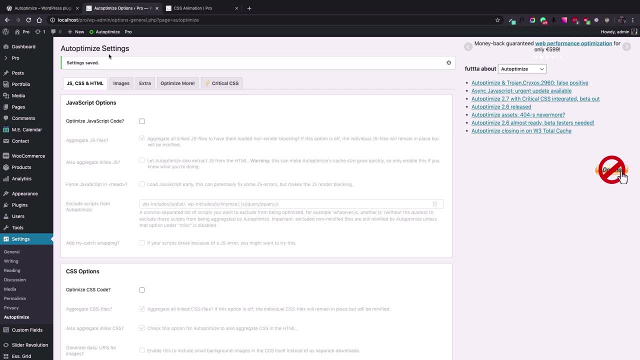 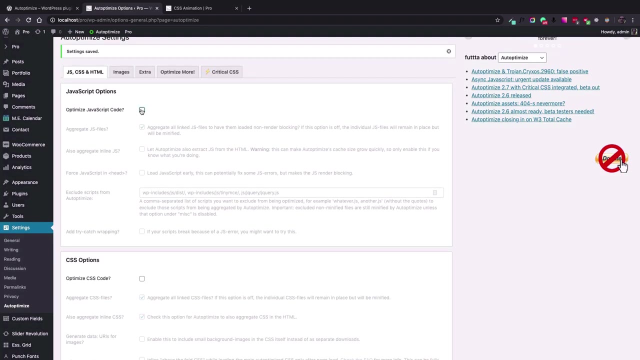 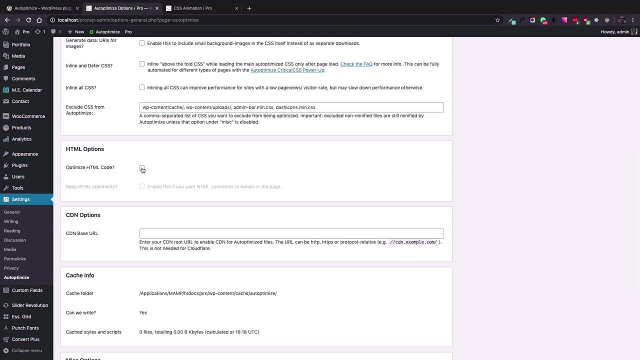 to access the auto optimize settings. For the first tab, we have the JS, CSS and HTML, which nearly is the most important tab of the auto optimize plugin settings. I simply just enable the java script code optimization, CSS code optimization And HTML. I'mma just create one for you. 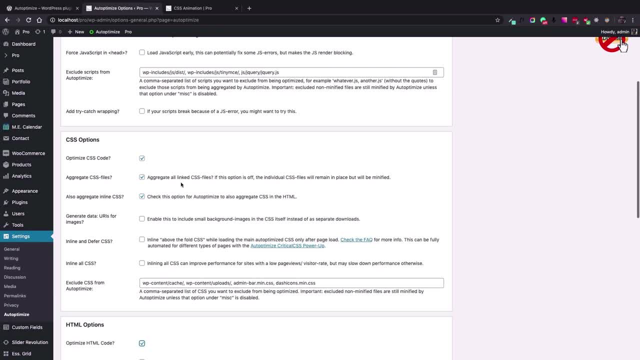 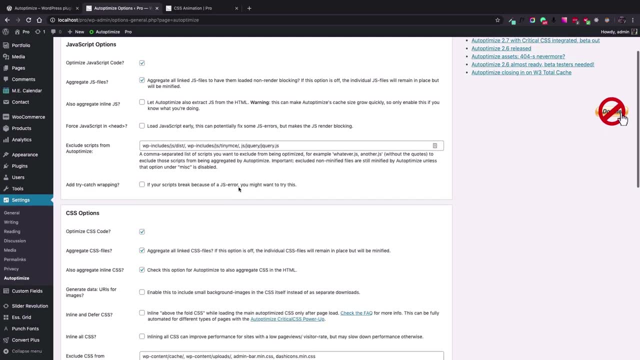 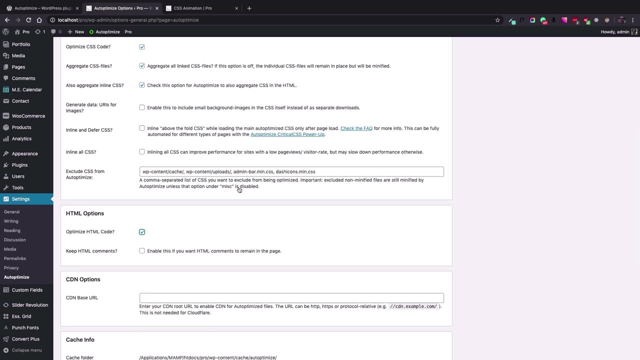 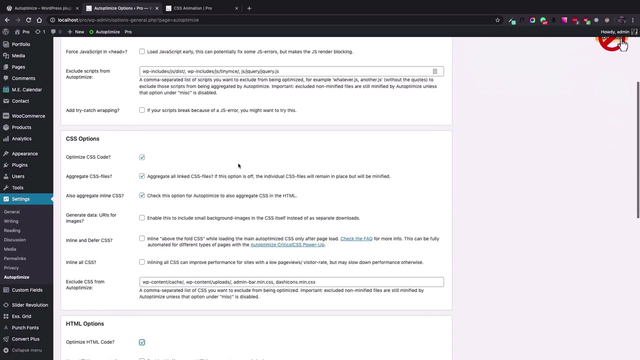 html code optimization. i will not touch anything else because if we want to go deeper and delve into all the details, it will take time and it is kind of very specific way to go and it is outside in the scope of our video here. so let's save the option and empty cache. 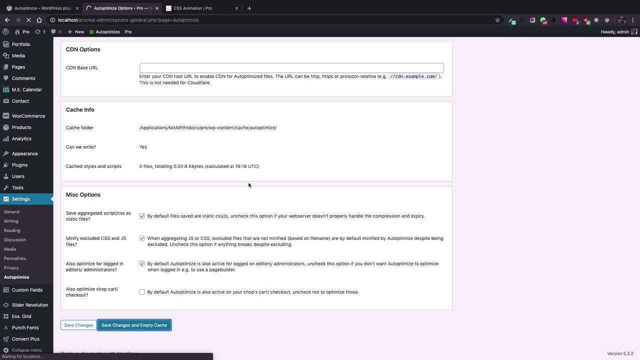 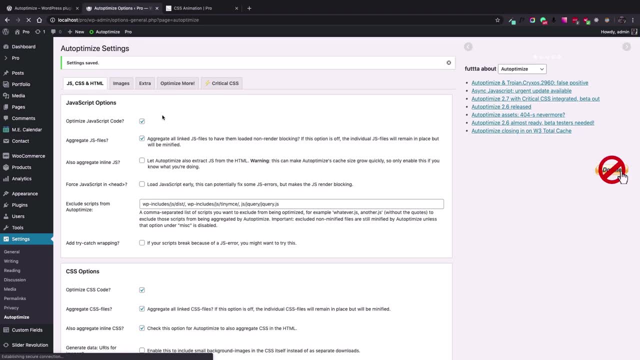 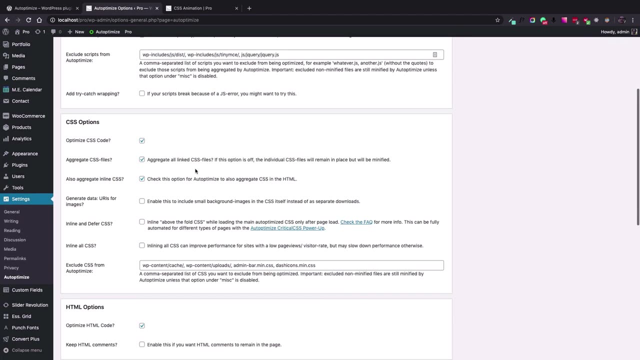 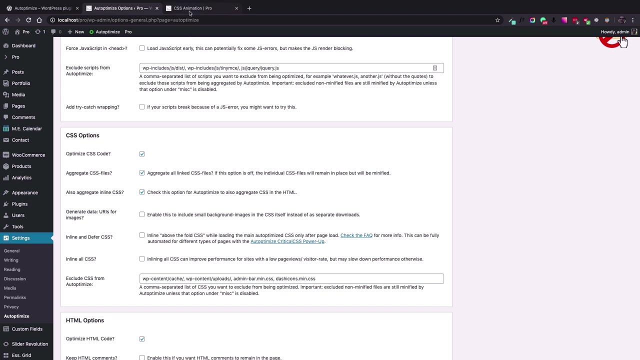 so the thing that auto optimize plugin now does is that it searches for all the javascript sources in the page and for the all the website and make sure that it minifies all the javascript css files and also merge them to one file. so if i reload the page now and check the page, 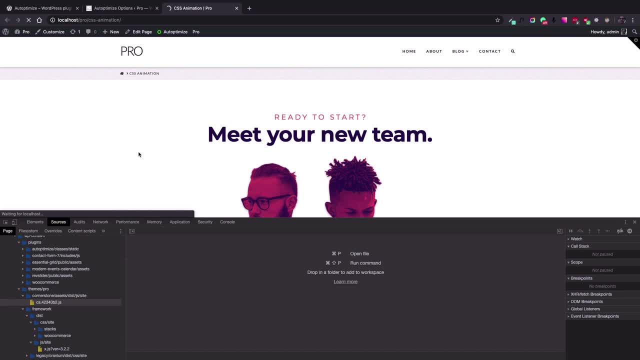 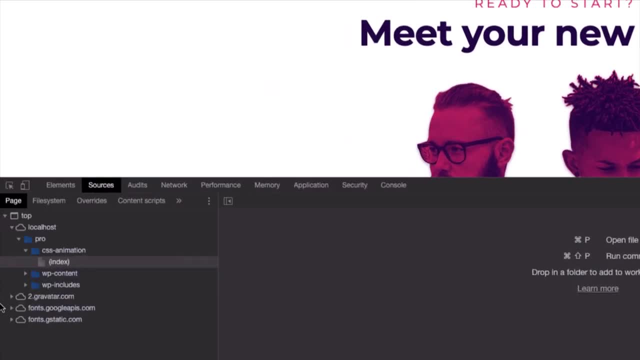 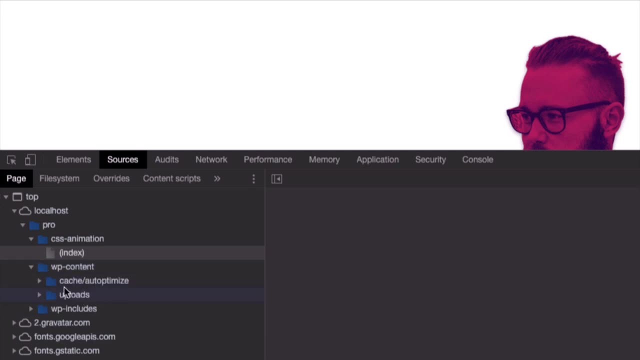 and it will show me that it's done. so let's go ahead and do that. so if i click the sources tab of the google chrome developer toolbar here now, if i go to wp content, you're gonna see that there is no plugin or theme folder anymore and there is a new folder called. 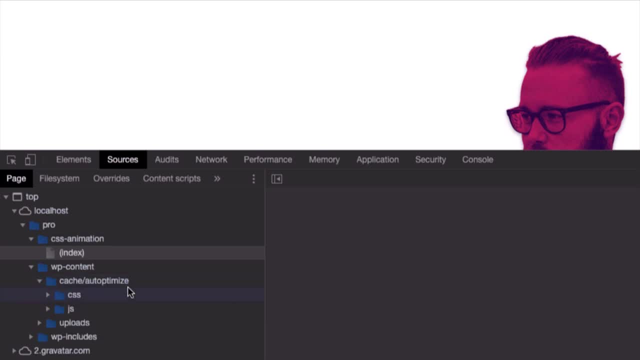 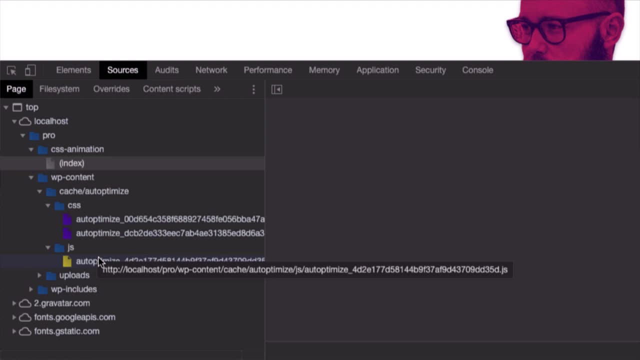 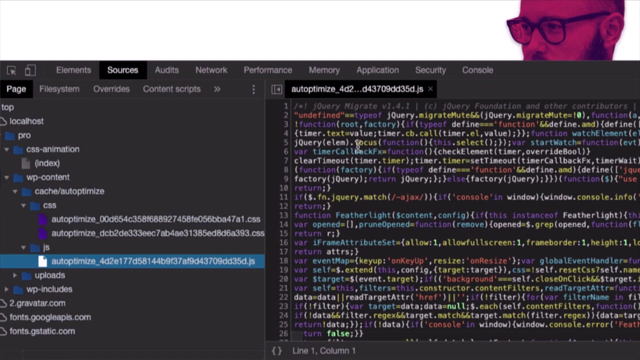 cache with the auto optimize subfolder, which includes just two css files and a javascript file. that's it. the javascript file is minified and all the other javascript files of different plugins are merged to one file and loaded them, and that will going to make a huge difference and cause the 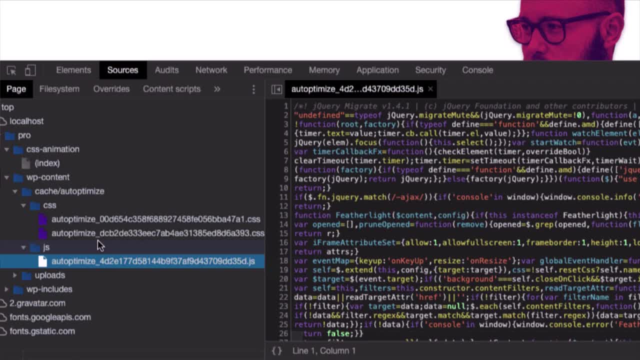 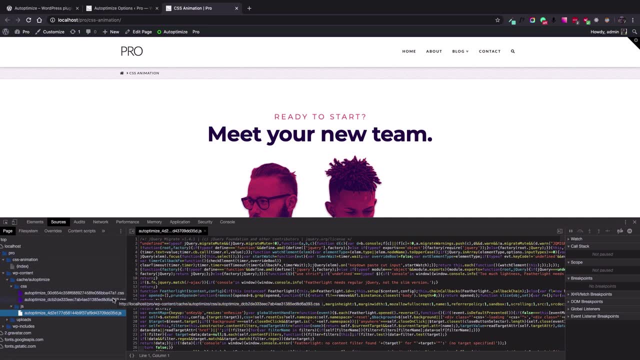 web page to load very quickly. so that's it. that is how you would just enable the minification and also the merging of the files to make sure that your page is super fast. but and also you should check the front end of the website and i have the page working correctly with no problem. but for any, 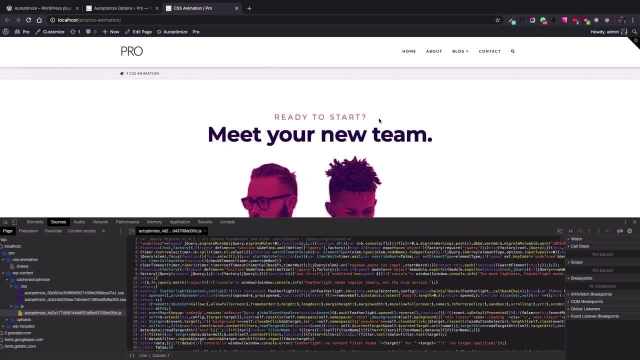 reason that you might see the front end of the website does not work. it might be caused by the merging or minification, and you need to just exclude the files of the theme or whichever plugin that you used and see that the result is not what you want to see. if you want to exclude the files from the 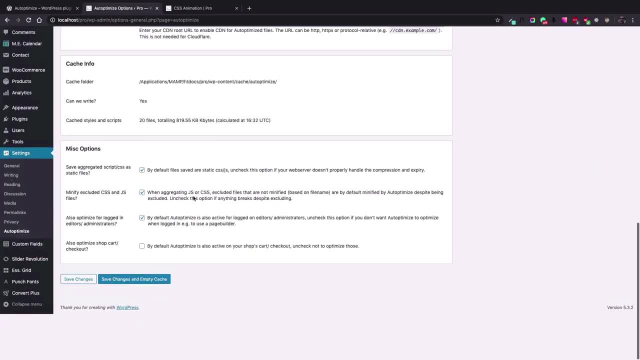 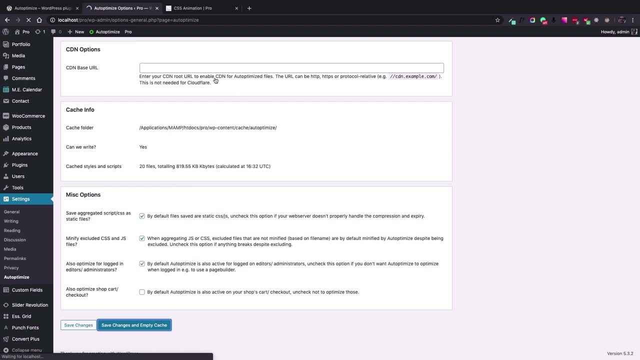 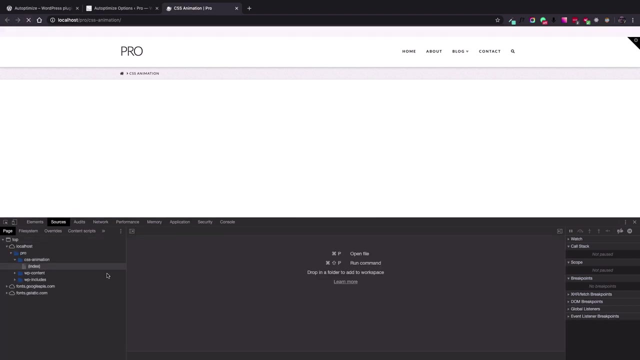 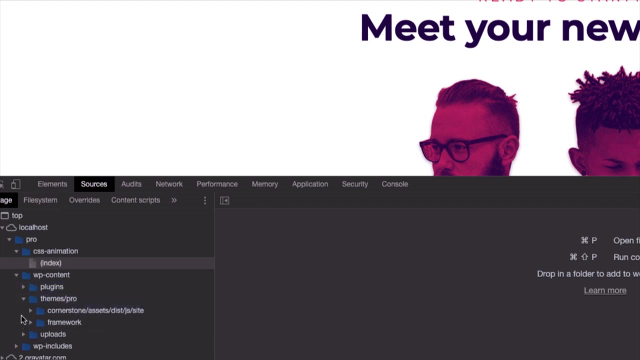 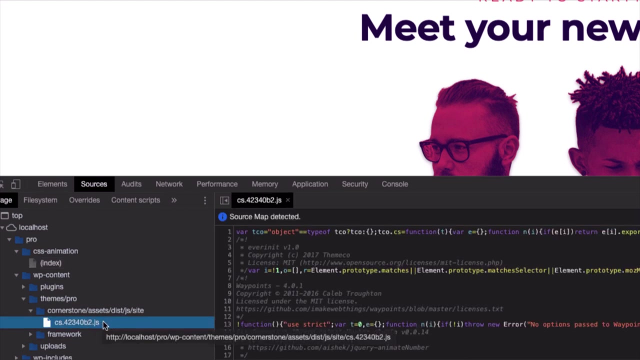 just process of the auto optimize plugin. i just disabled the settings to go back and see the original files that were loaded. so i can make sure that i, for example, for our theme, i'm going to just use the address of this file, the js file that the theme loads. how i should just retrieve the address is to just select the file. 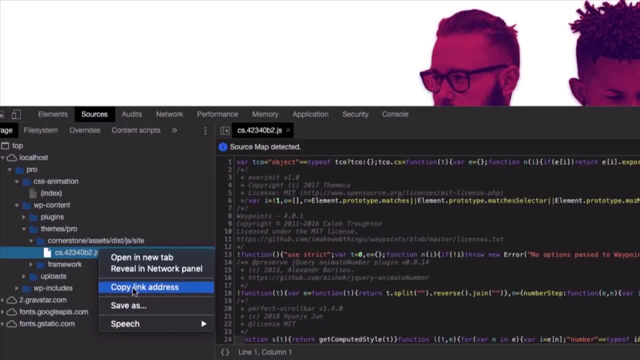 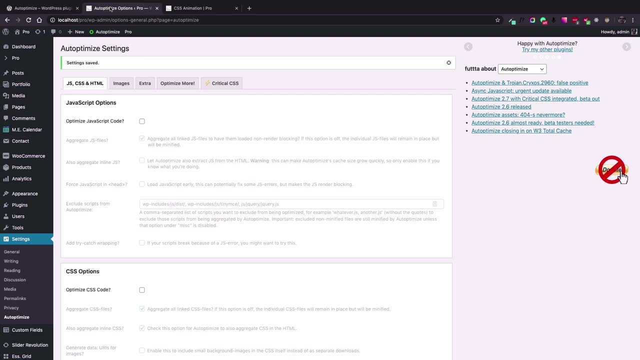 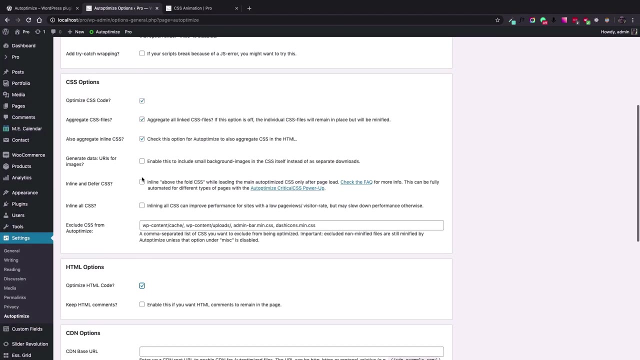 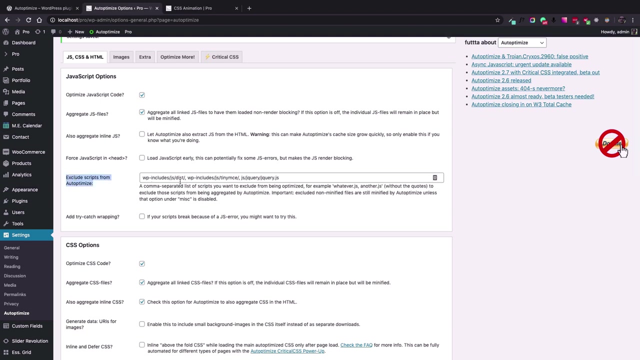 and right click on the file and select the copy link address. okay, and then in the auto optimize options, which i am going to re-enable again, we have a section for the javascript files that we can exclude the scripts. the way that it works is a comma separated list. 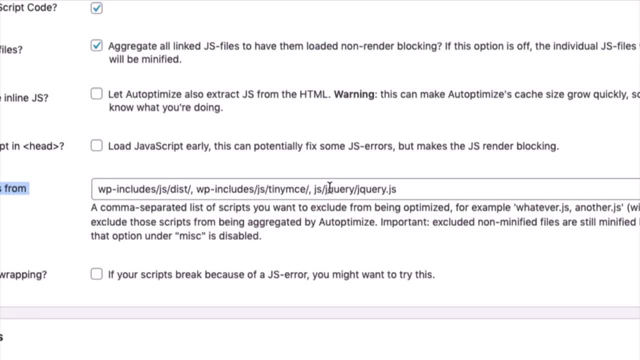 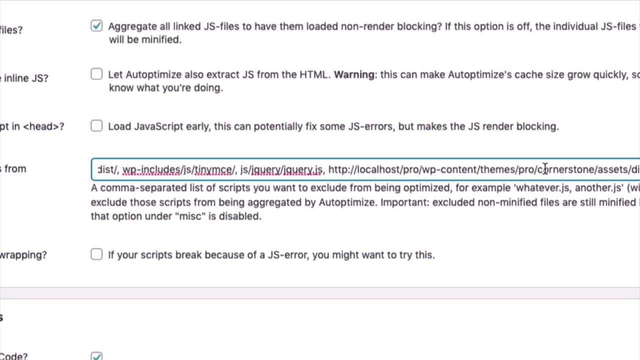 that you can add whatever javascript file that you want to exclude from the optimization. so i just add another comma and paste the url at the address that i've copied, but the address should start from the root of the wordpress installation. for me the root started from the wp content and the rest is. 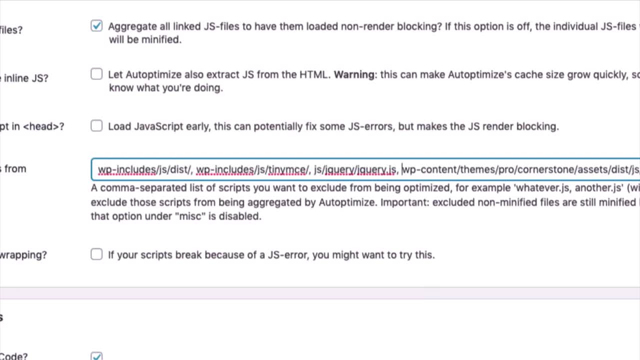 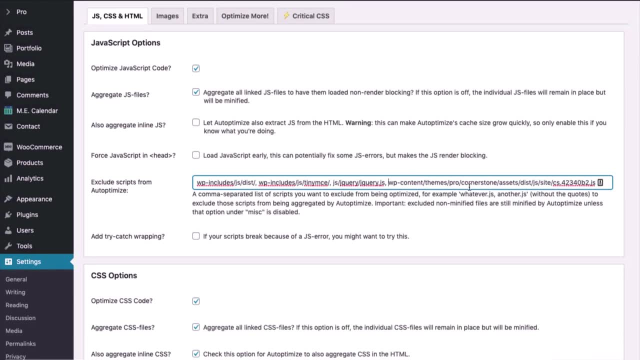 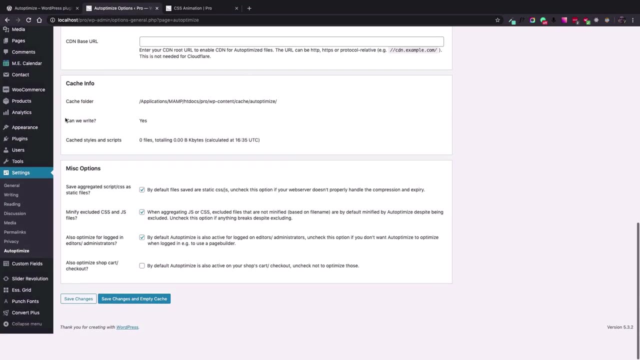 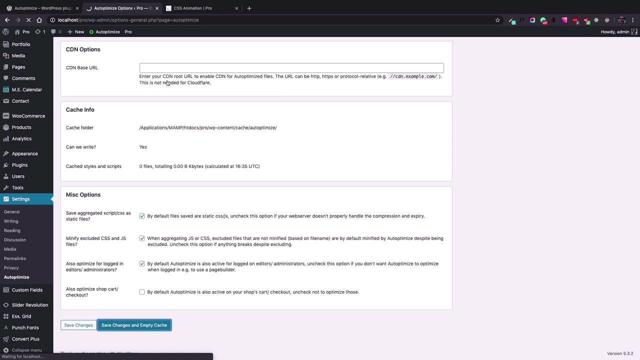 the main domain for my local installation, which i am going to just delete. so we have now wp content themes, blah, blah to the end, which is the script that i want to exclude. so let's again save changes and empty cache and reload the page on the front end of the website. 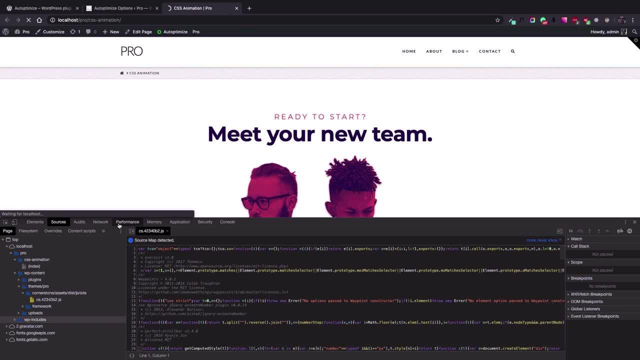 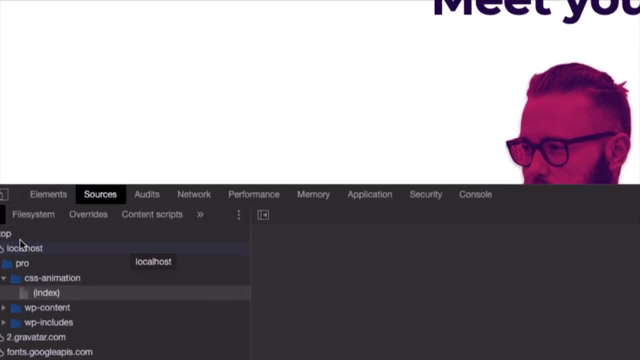 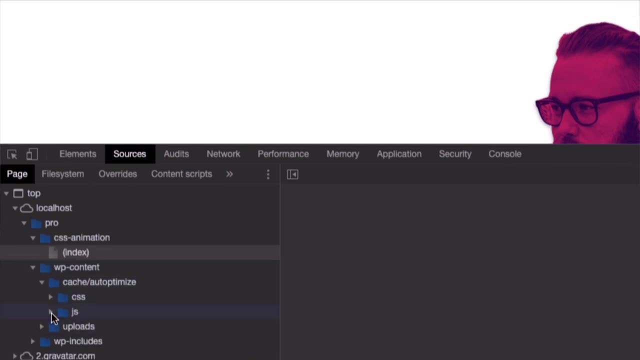 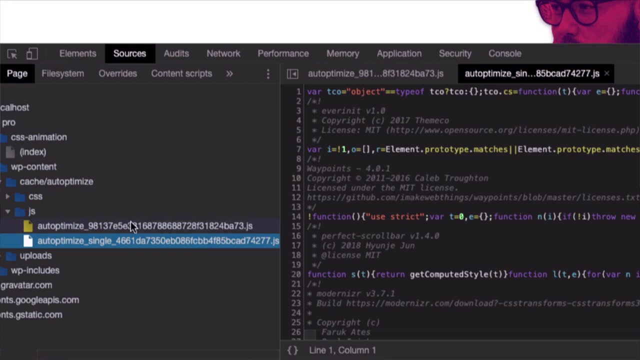 and check the google chrome browser developer toolbar to see how excluding our javascript file worked. so now, if i go to wp content, i'm going to see: uh, just two javascript files, and beforehand we had just one. and this is the first one. the last one is exactly the javascript file that we excluded. that is why it shows separately. 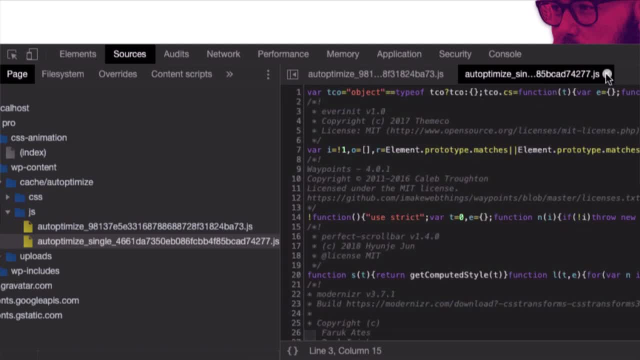 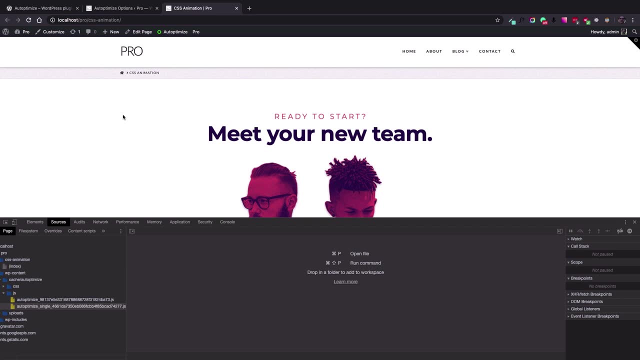 without the minified version. this is how we exclude the file from the optimization. the last point is that optimizing a page is something that we should do after the development of the website, so make sure that you will do the optimization after you did all the changes that.